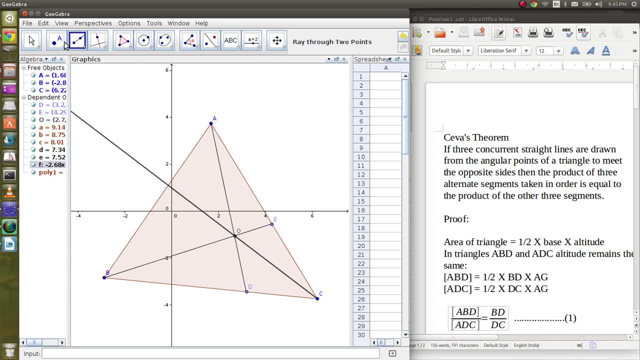 This is it, and let's take it as F. Okay, so the theorem is: alternate segments, as in suppose AF into BD into CE equals AE into CD into BF. Okay, let's show this by colouring the segments. it would be easy to understand then. 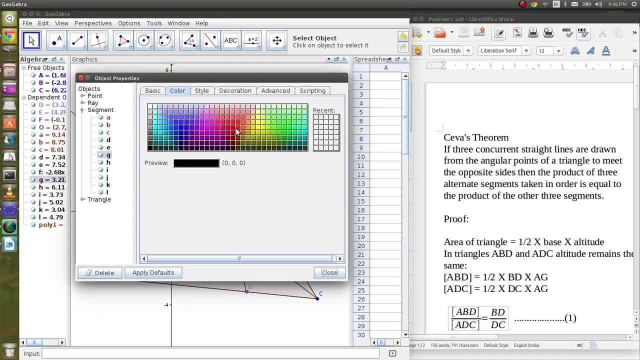 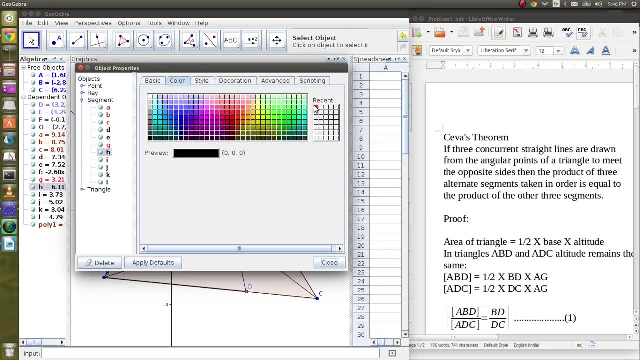 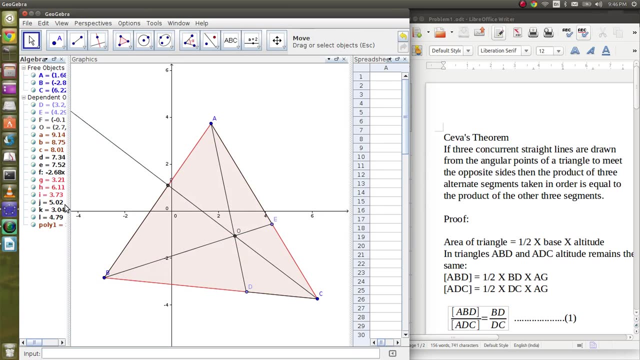 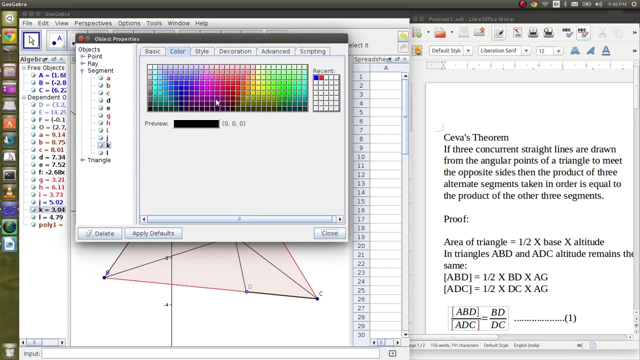 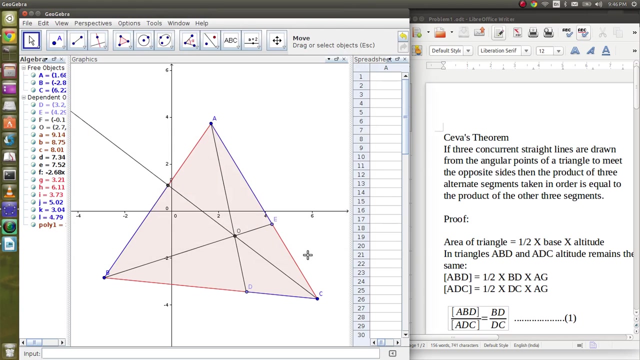 Okay, after properties, I will colour this red, This again is red, and this too Done, and I will colour the other segments in blue. Okay, Okay, That's it. So the theorem is: the product of the segments coloured in red is equal to the product of 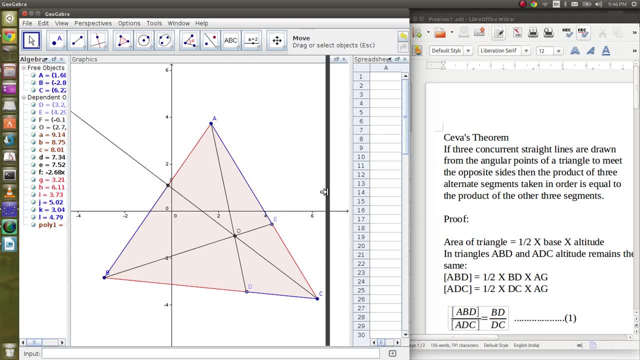 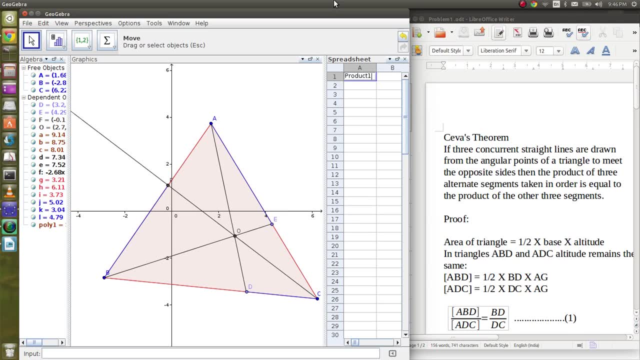 the segments coloured in blue. I will show explain this with the help of a spreadsheet. Okay, let the product of segments in red be product one and that in blue be product two. Oops, Sorry. Okay, now this is G into H into I is something. and this is also G into H into I. 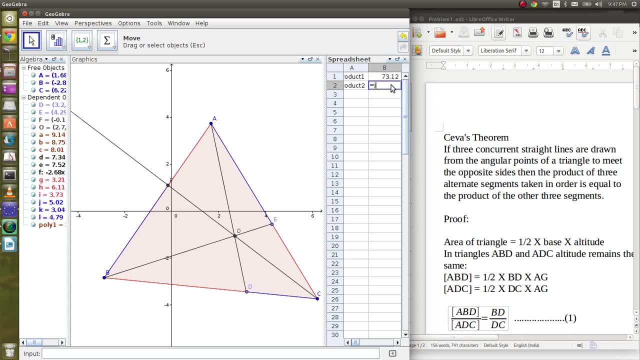 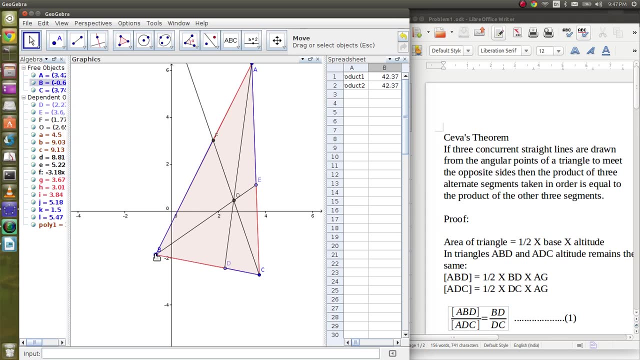 Sorry, J into K into L, This comes out to be same. Let's move it around a bit. Okay, Let's move it around a little to prove my point. See, this comes the same always. Okay, now I will move on to the proof of this theorem. 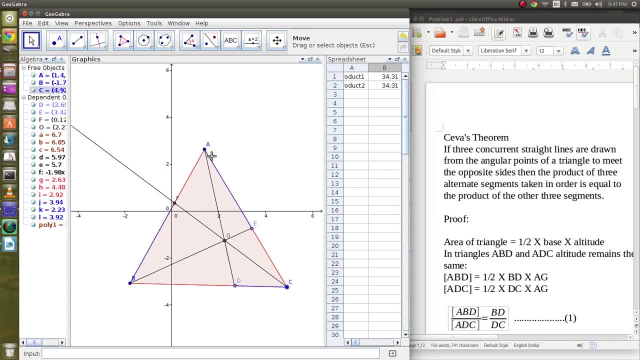 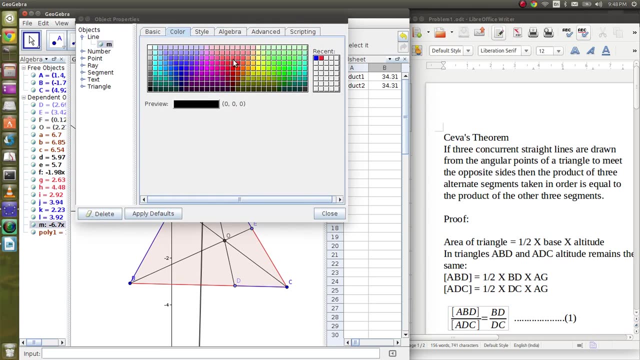 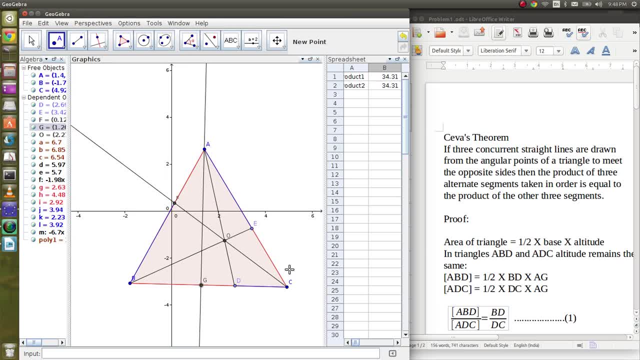 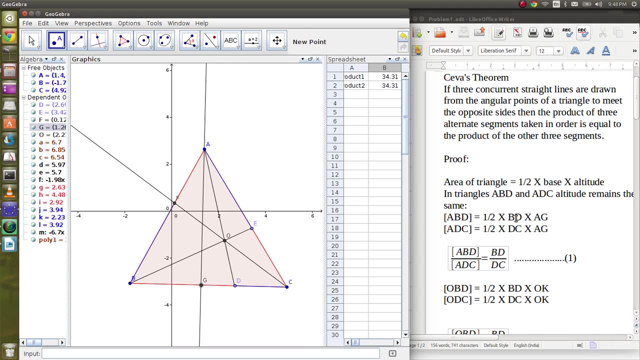 Okay, Okay, I have named it G. Okay, So the area of triangle ABD is half s into height, which is the height is AG and the base is BD. So the area of triangle ABD is half into BD, into AG, And the area of triangle ADC. the height remains the same, and so the area of triangle ADC remains. 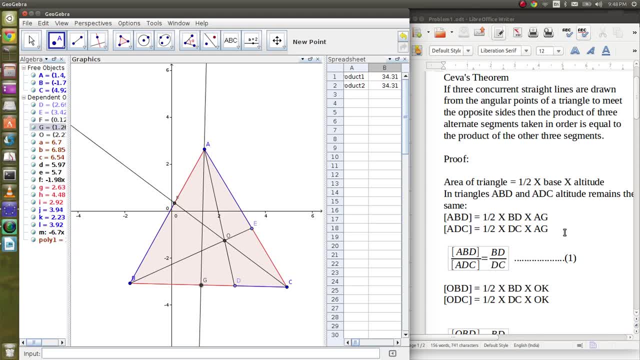 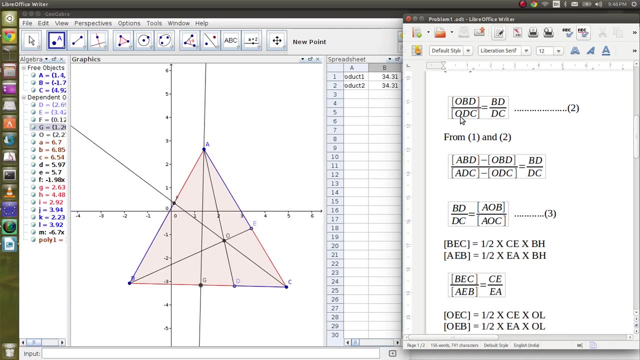 is the same. So the area of triangle ADC is half into DC, into AG. So when we divide the area of triangle ABD by area of triangle ADC, we get BD by DC. Okay, So now let us consider triangle OBC. I will delete this line. This is not needed anymore, Deleted. Now let us 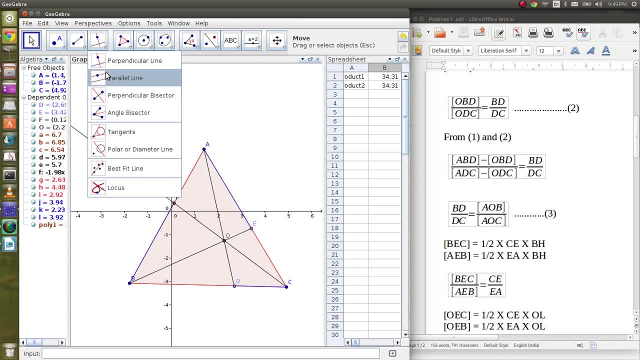 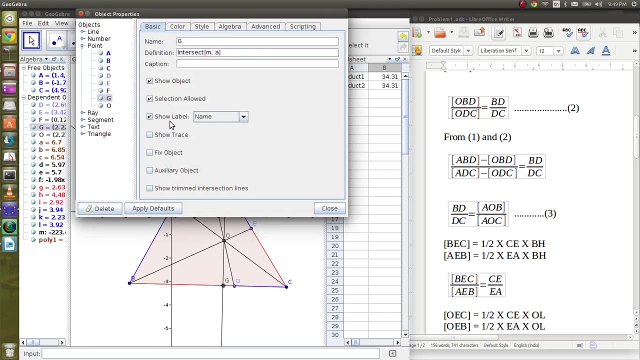 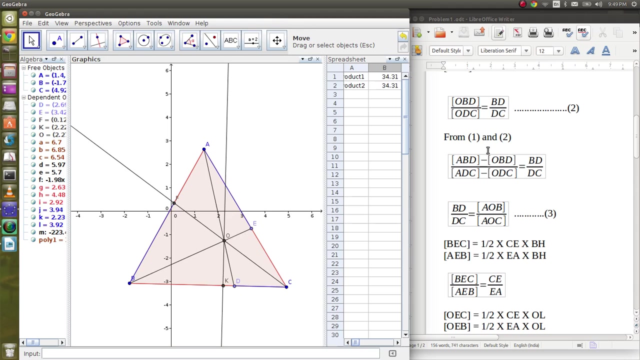 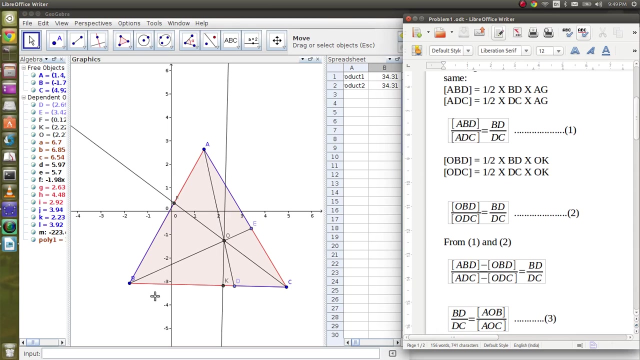 drop a perpendicular from O to BC. That is it. Let us name it K. This is K. Okay. So triangle OBD – the area of triangle OBD is half into BD into OK, and triangle ODC is half into DC into OK. 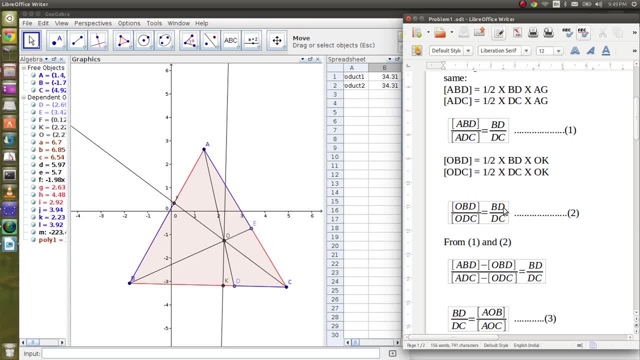 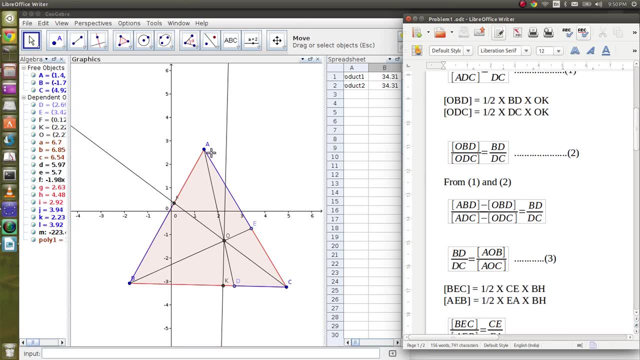 Similarly, the area of triangle OBD is half into BC into K. So triangle OBD is half into BC into OK. because the area of triangle OBD is half into BC into K You denote, Performing the ratio of these two area comes out to be BD by DC, as the others cancel out. ok now from. 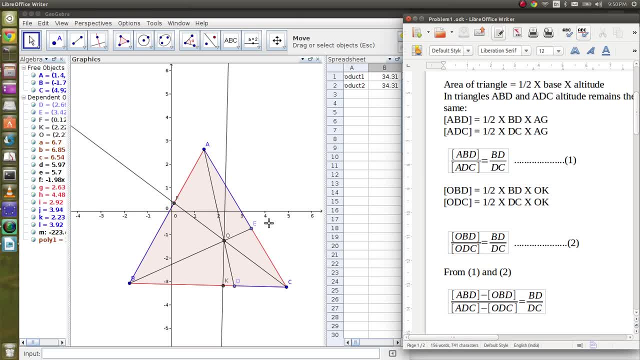 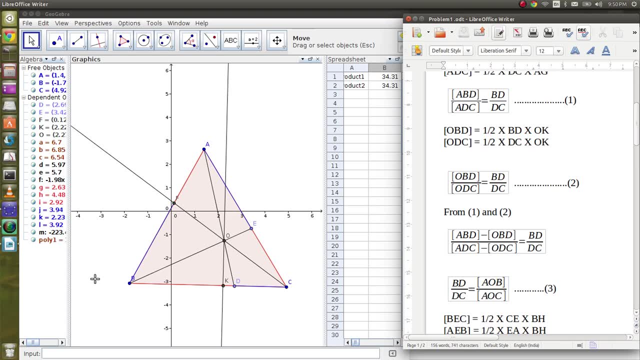 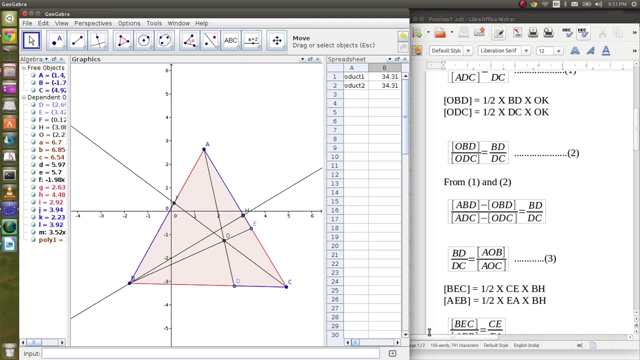 number one and number two. if we subtract the areas, we get this. so this is AOB by AOC, is BD by DC. this one, ok. now let's drop the altitude from B to AC. now let's name it H, ok, ok. ok now in triangle AAB and EBC, the area of triangle AAB is half into EA, into BH. the altitude, 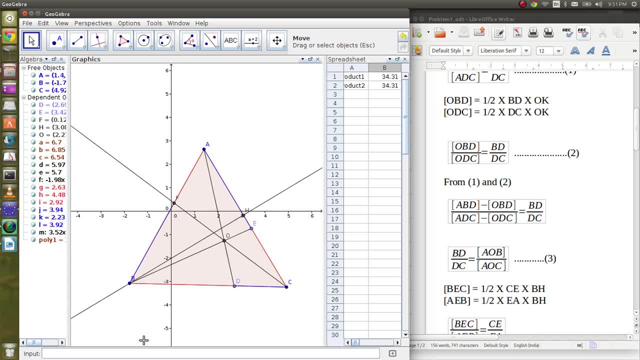 ok, ok, ok, ok, ok. so now that we know this, we can check this. then theña Earl decreta is BEC by C. when this has EBC comes out to be half into ec, into BH, the altitude. so now come back again there. there is no difference in the area of triangle. 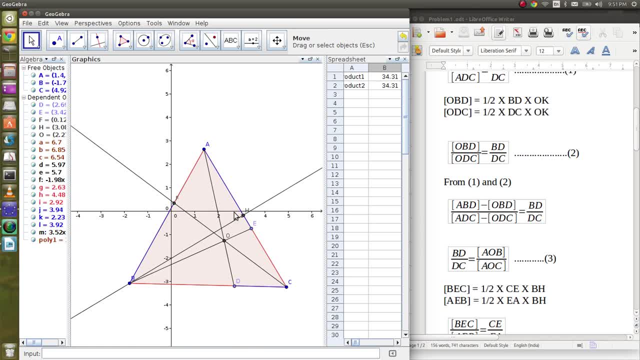 ok, ok, ok, ok, so one больше Hadi. so the y ratio will be same as exercised this one. so here we divide theilibrium as number 2, so we get 3 times. this is the value fed s in and the area of triangle BEC. this one is half into EC, into BH, the altitude again. so 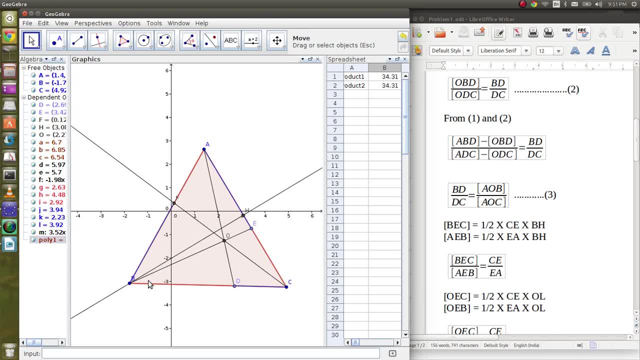 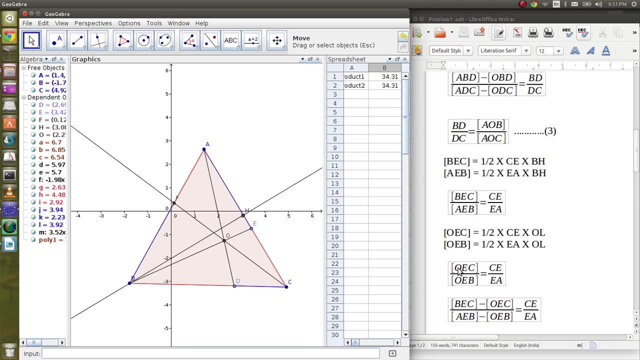 now again, if divide this, we get BEC by AAB equals to CE by EA. BEC by AAB is CE by EA. similarly, if we draw a perpendicular from o on ac, will compensation will be equal to AC. we would get OEC by OAB equals to CE by EA. again, if you subtract the areas we